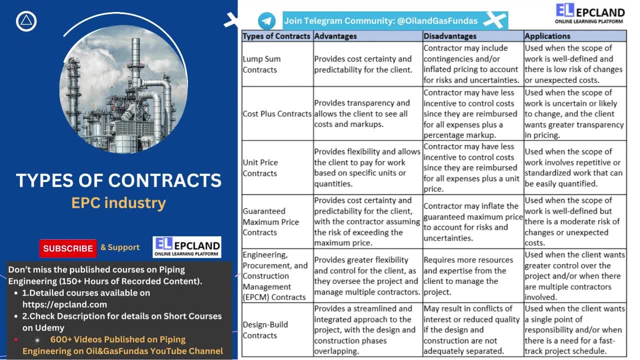 much they will be paying for the project and can budget accordingly. This can be particularly important for clients with limited budgets or tight project schedules. However, there are also disadvantages to lumpsum contracts Because the contractor assumes the risk of unexpected costs or changes to the scope of work. they may include contingencies and or inflated pricing in the 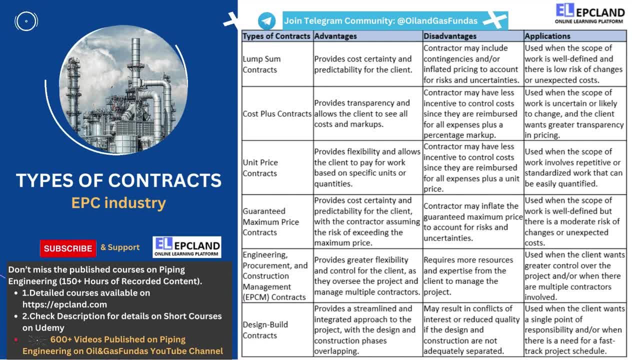 lumpsum to account for risks and uncertainties. This can result in higher overall costs for the client. Overall, lumpsum contracts are best suited for projects with a well-defined scope of work and a low risk of changes or unexpected costs. They can provide cost certainty and predictability. 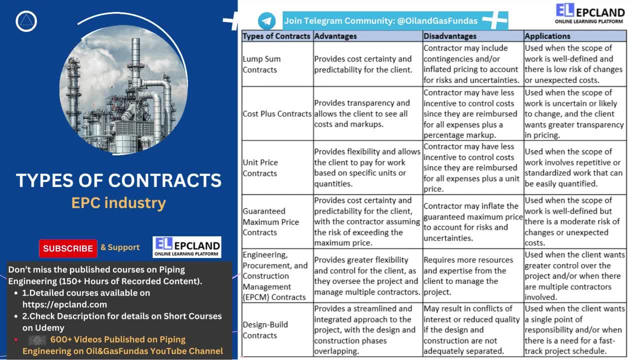 for the client, but may result in higher overall costs if the contractor includes contingencies and or inflated pricing to account for risks and uncertainties. As with any type of contract, it is important to carefully consider the specific terms and conditions of a lumpsum contract before. 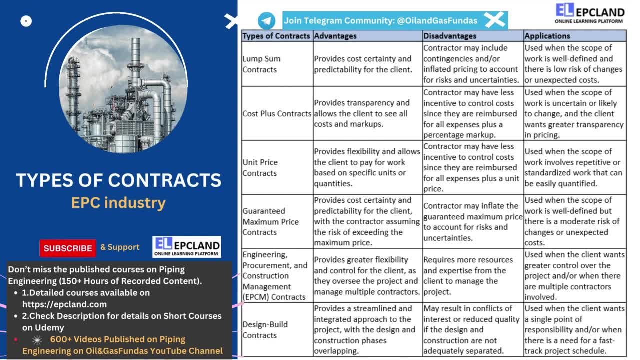 entering into it. Let's proceed to the second type of contract mentioned in the table. Cost-plus contracts are another type of contract commonly used in the engineering, procurement and construction EPC industry. They are typically used when the scope of work is uncertain or likely to change. 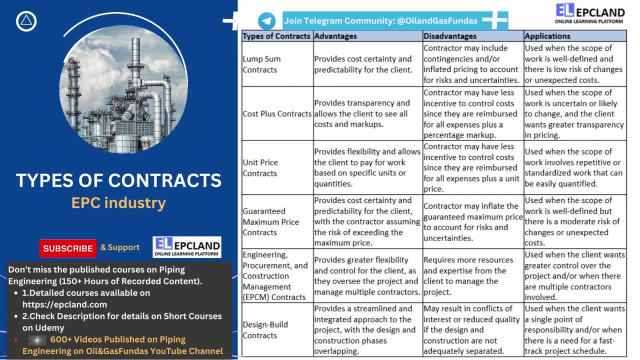 and the client wants greater transparency in pricing. One of the main advantages of a cost-plus contract is that it provides transparency and allows the client to see all costs and markups. With a cost-plus contract, the client is responsible for reimbursing the contractor. 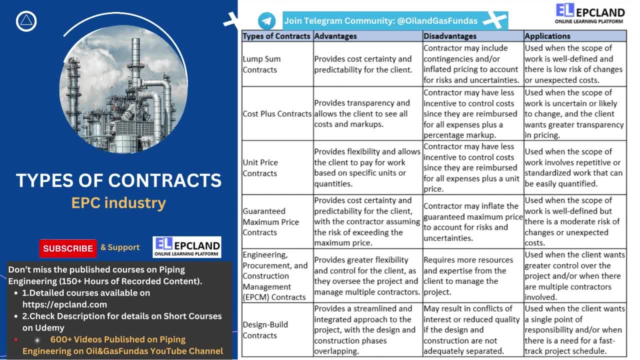 for all expenses, including labor, materials and overhead costs, plus a percentage markup. This can provide greater transparency in pricing and help the client to better understand the costs associated with the project. However, there are also some potential disadvantages to cost-plus contracts, Because the contractor is reimbursed for all expenses plus a percentage markup. 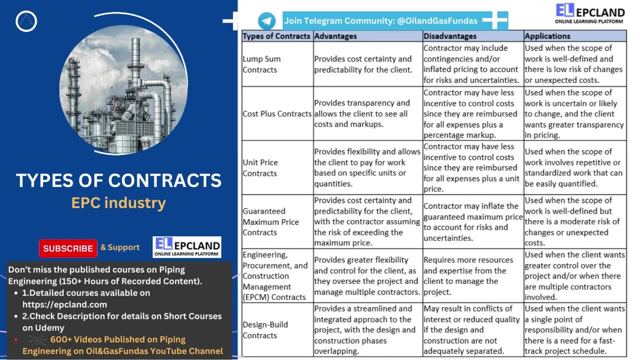 they may have less incentive to control costs. This can result in higher overall costs for the client. Overall cost-plus contracts are best suited for projects that are more expensive, with an uncertain scope of work or a high risk of changes. They can provide greater 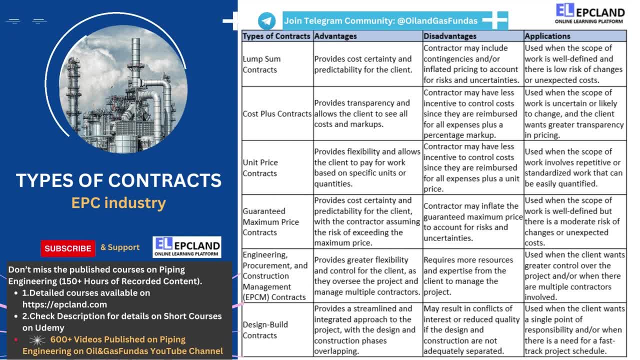 transparency in pricing and help the client to better understand the costs associated with the project. However, they may result in higher overall costs if the contractor does not effectively manage costs. As with any type of contract, it is important to carefully consider the specific terms and conditions of a cost-plus contract before entering into it. The following contract: on the list is the first one. The subject that is used in a cost-plus contract is the secondAll contract on the list. The subject that is used in a cost-plus contract is the thirdall contract on the list. The subject that is used in a cost-plus contract is the thirdall. 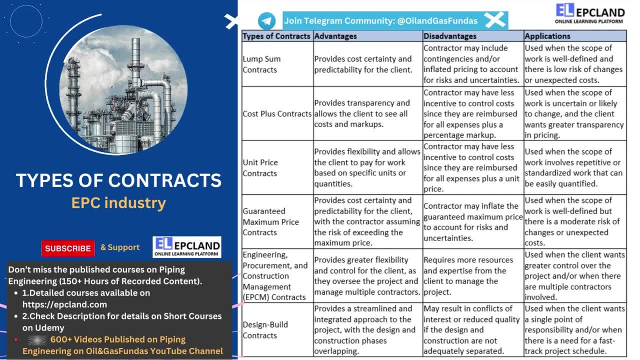 third one, which is unit price contracts. Unit price contracts are another type of contract commonly used in the engineering, procurement and construction EPC industry. They are typically used when the scope of work involves repetitive or standardized work that can be easily quantified. 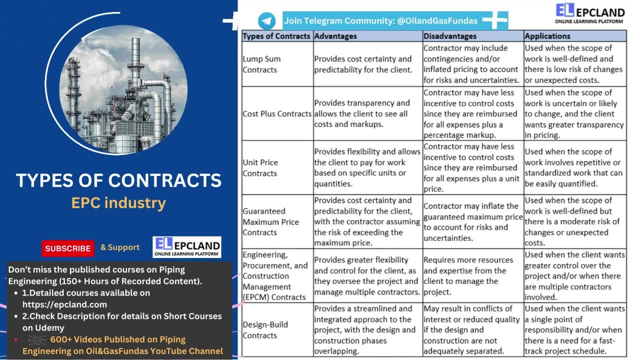 One of the main advantages of a unit price contract is that it provides flexibility and allows the client to pay for work based on specific units or quantities. With a unit price contract, the client pays the contractor a predetermined unit price for each unit of work completed. This can be particularly useful for projects with a large number of similar 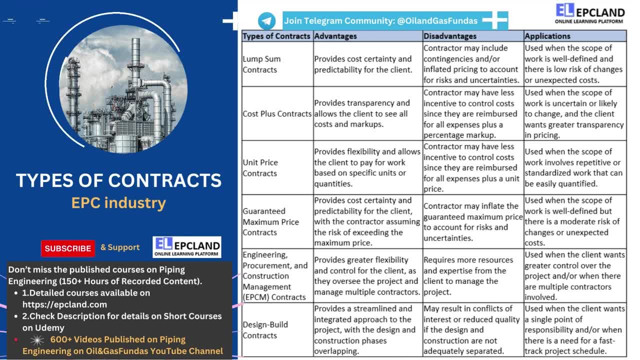 tasks, as it allows the client to easily adjust the scope of work as needed. However, there are also some potential disadvantages to unit price contracts. Because the contractor is reimbursed for all expenses plus a unit price, they may have less incentive to control contracts. 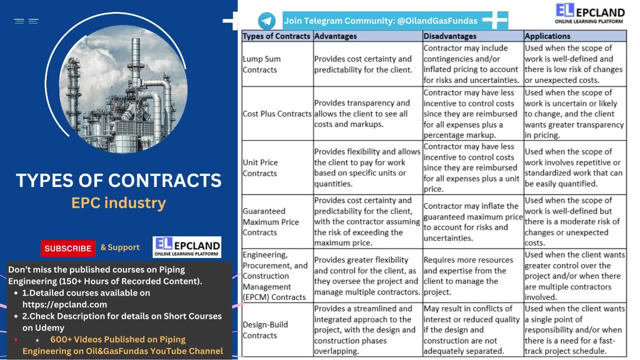 This can result in higher overall costs for the client. Overall unit price contracts are best suited for projects with repetitive or standardized work that can be easily quantified. They can provide flexibility in pricing and help the client to better manage the scope of work. However, they may result in higher overall costs if the contractor 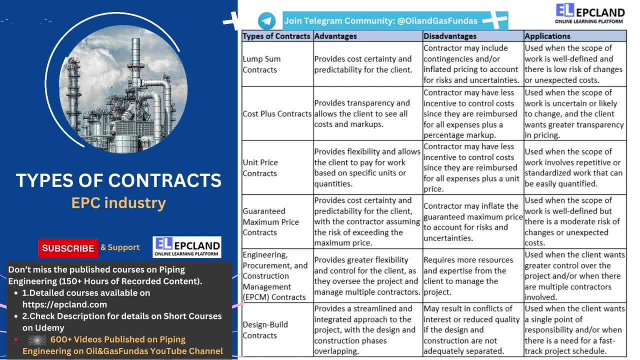 does not effectively manage costs. As with any type of contract, it is important to ensure that the contractor is able to manage the costs of the project. It is important to carefully consider the specific terms and conditions of a unit price contract before entering into it. Next up, we have the fourth contract. 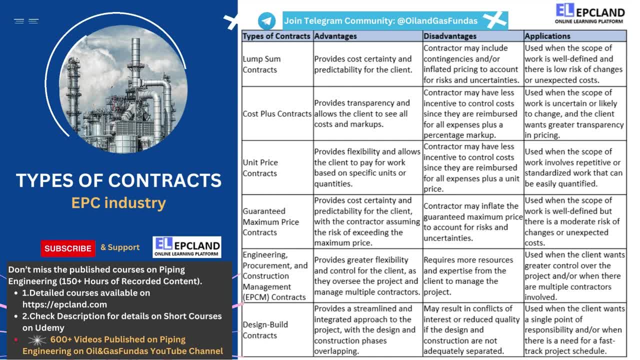 Guaranteed Maximum Price- GMP Contracts. These contracts are another type of contract commonly used in the engineering procurement and construction EPC industry. They are typically used when the scope of work is well-defined, but there is a moderate risk of changes or unexpected. 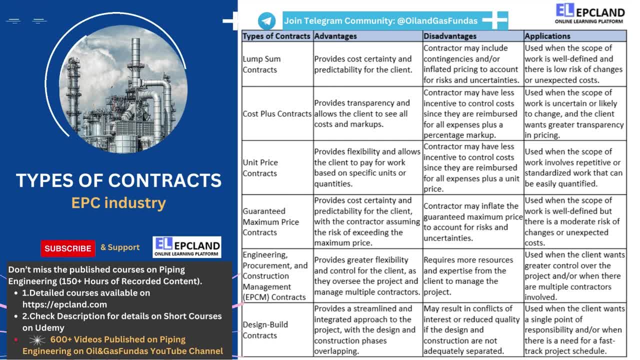 costs. These contracts are used when the scope of work is well-defined, but there is a moderate risk of changes or unexpected costs. One of the main advantages of a GMP contract is that it provides cost certainty and predictability for the client, with the contractor assuming the risk of exceeding. 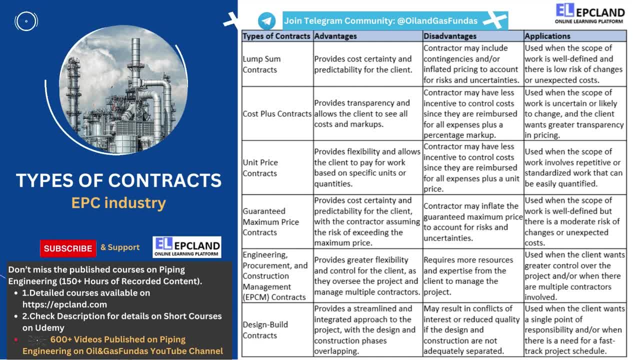 the maximum price. With a GMP contract, the contractor agrees to a maximum price for the project, which provides the client with the assurance that the project will not exceed a certain cost. However, the contractor also has an incentive to keep costs down in order to increase. 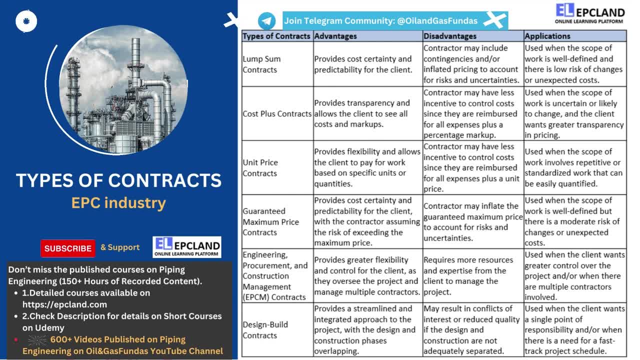 their profit margin. However, the contractor also has an incentive to keep costs down in order to increase their profit margin. However, there are also some potential disadvantages to GMP contracts, Because the contractor assumes the risk of exceeding the maximum price they may inflate. 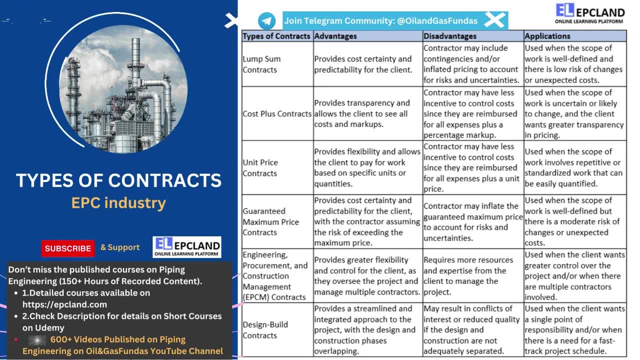 the guaranteed maximum price to account for risks and uncertainties. This can result in higher overall costs for the client. Overall, GMP contracts are best suited for projects with a well-defined scope of work but a moderate risk of changes or unexpected costs. They can provide cost certainty. 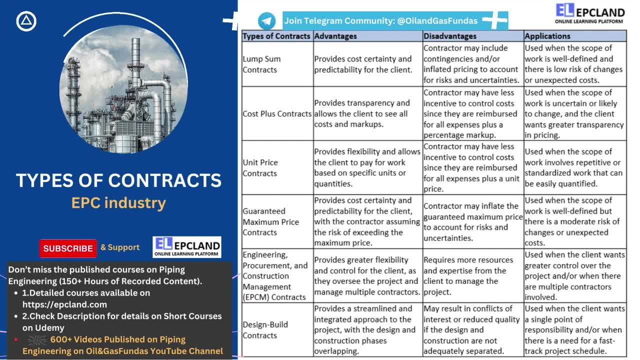 and predictability for the client, while also incentivizing the contractor to keep costs down. However, they may result in higher overall costs if the contractor inflates the guaranteed maximum price. As with any type of contract, it is important to carefully consider the specific 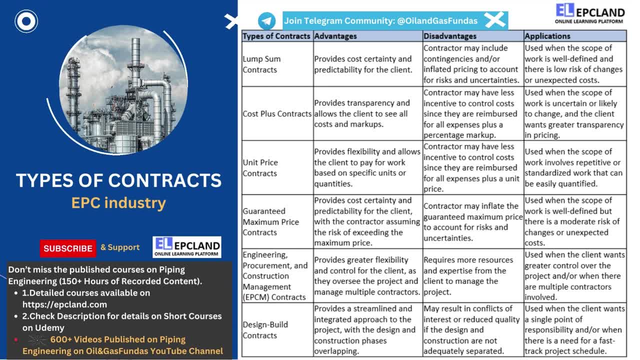 terms and conditions of a GMP contract before entering into it. Okay, now let's move to next contract of this session: Engineering Procurement and Construction Management, EPCM. These contracts are a type of contract commonly used in the engineering procurement. 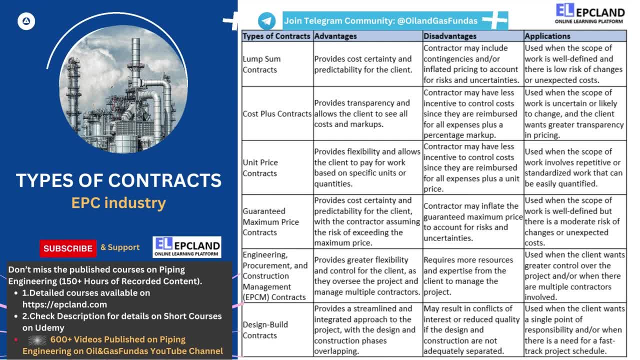 and construction EPC industry. They are typically used when the client wants greater control over the project and or when there are multiple contractors involved. One of the main advantages of an EPCM contract is that it provides greater flexibility and control for the client. With an EPCM contract, the client oversees the project and manages multiple 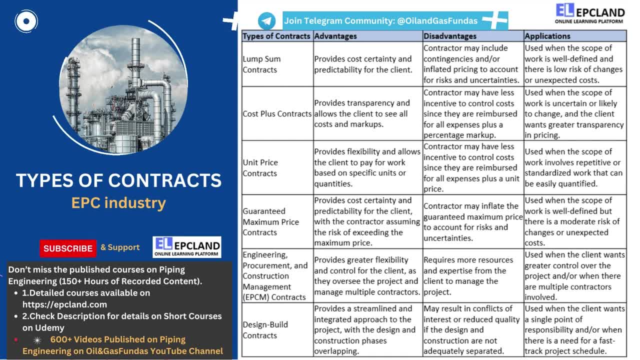 contractors, which allows them to have greater input and control over the project. Additionally, because the client manages the project themselves, they can potentially save money by avoiding markups that would be charged by a general contractor. However, there are also some potential disadvantages to EPCM contracts. Because the client manages the project themselves, 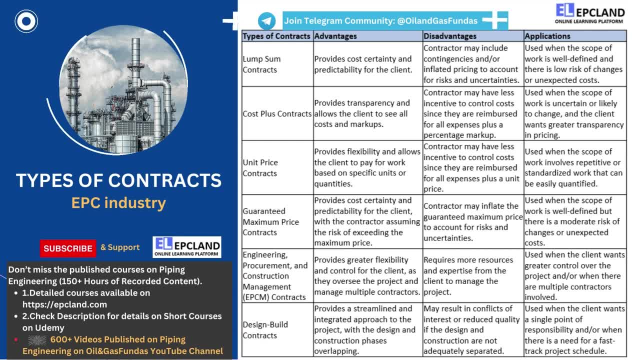 it requires more resources and expertise to effectively manage the project. This can be challenging for contractors, Clients who are not experienced in project management or who do not have sufficient resources to manage the project effectively. Overall, EPCM contracts are best suited for clients who want greater control over the project and who have the resources and expertise to manage. 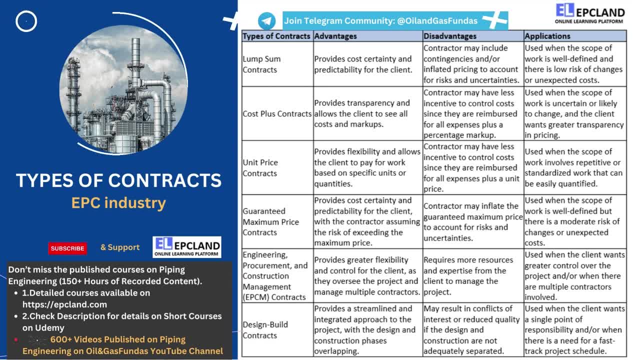 the project effectively. They can provide flexibility and potentially save money by avoiding markups charged by a general contractor. However, they require more resources and expertise from the client to manage the project. This can be challenging for contractors. However, they require more resources and expertise to manage the project effectively. As with any type of contract, 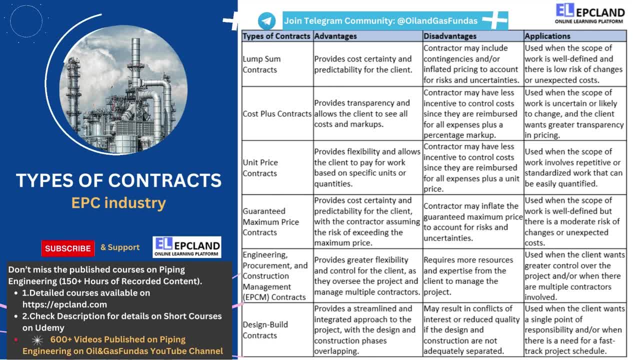 it is important to carefully consider the specific terms and conditions of an EPCM contract before entering into it. Okay, now let's move to last contract of this session: Design-Build Contracts. These are a type of contract commonly used in the engineering, procurement and construction EPC. 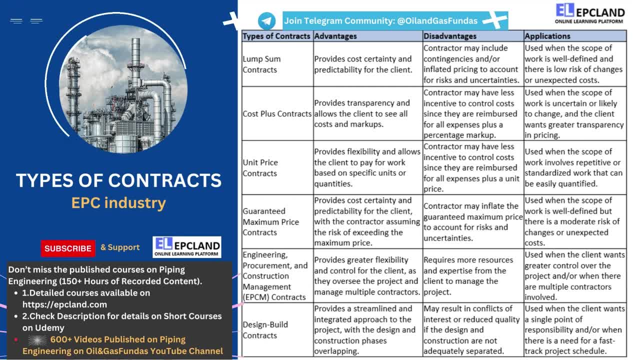 industry. They are typically used when the client wants a single point of responsibility and or when there is a need for a fast-track project schedule. One of the main advantages of a Design-Build Contract is that it provides a streamlined and integrated approach to the project. 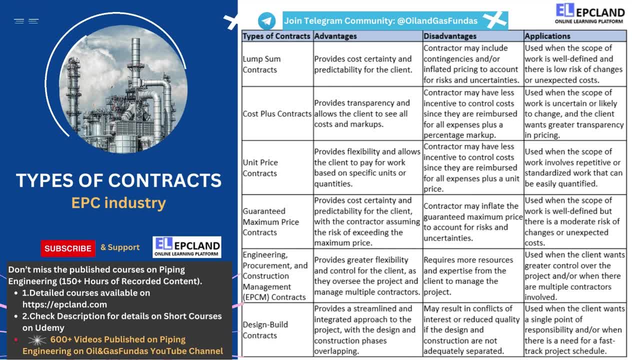 With a Design-Build Contract, the design and construction phases of the project overlap, which can result in faster project completion times and potentially lower costs. Additionally, with a single point of responsibility, the client does not have to manage multiple contractors, which can simplify the project. 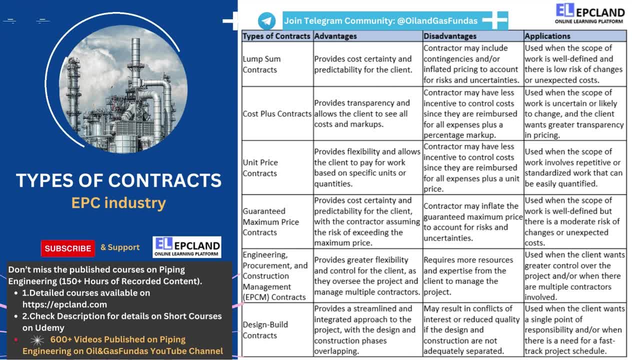 However, there are also some potential disadvantages to Design-Build Contracts Because the design and construction phases overlap. it can result in conflicts of interest or reduced quality if the design and construction are not adequately separated. Additionally, the contractor may have less incentive to control costs, since they are